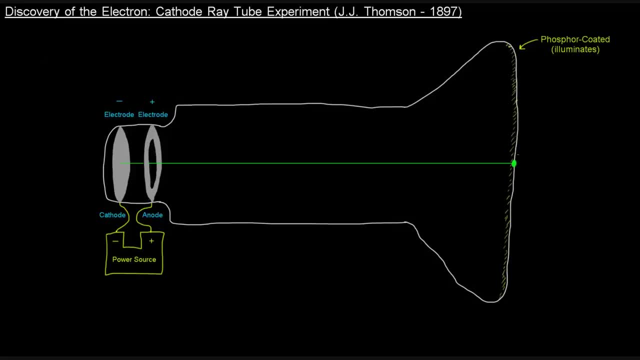 And it causes a little glow at this end of the tube because of the special coating on the inside of the tube. It's a phosphor coating, So it lights up. So Thompson sees this and he thinks: okay, what is this tube? 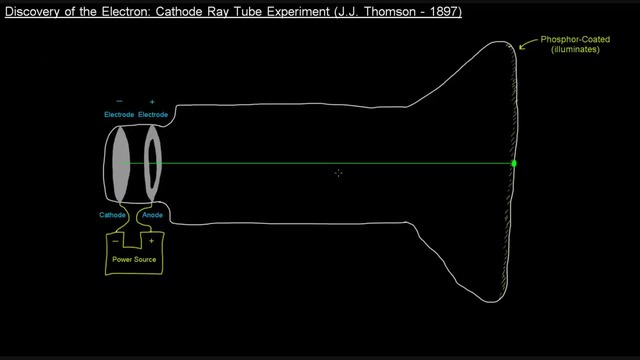 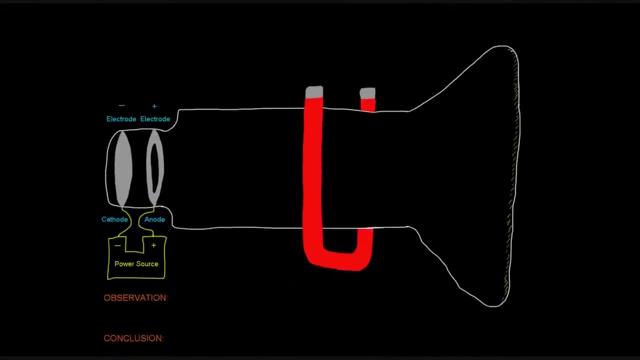 Of course, what is this tube's ray? What is this ray made up of? What is this beam made up of? And he thinks and wonders, okay, does this thing have a charge of some sort, an electrical charge? So what he does pretty genius: he grabs a magnet and he holds it kind of around the tube. 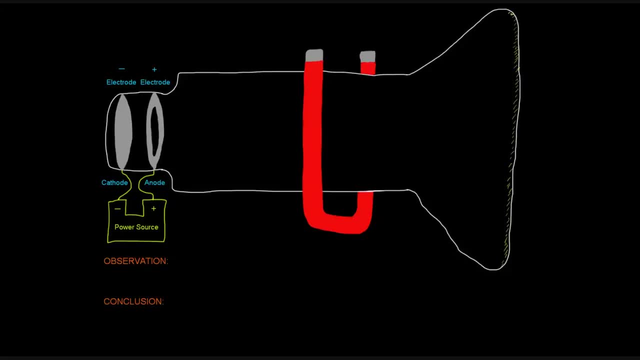 And he tries to see what's going on with the ray if this affects it. And so what he notices is: What he notices is that the beam bends, the ray bends in this magnetic field. That's the observation that he makes: The ray bent in a magnetic field. 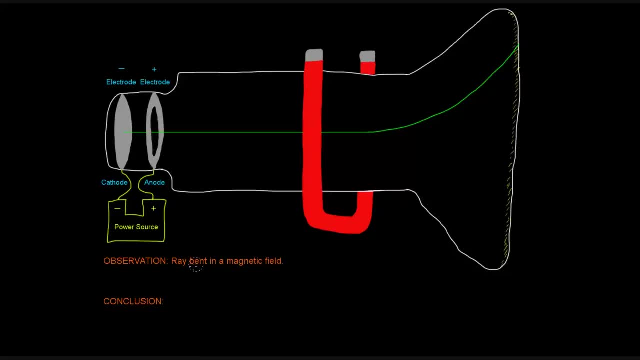 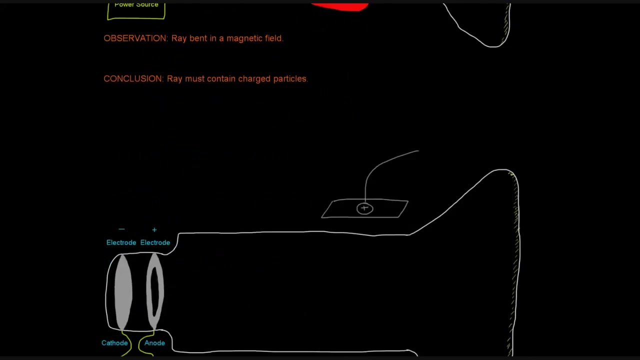 So his conclusion was that, because this ray bent in this magnetic field, that this ray must contain charged particles, Because something that's charged will bend in a magnetic field. So then he wonders: okay, What charge is this? So then what he does is he takes two plates, two metal plates, one of them being positively charged and one of them being negatively charged. 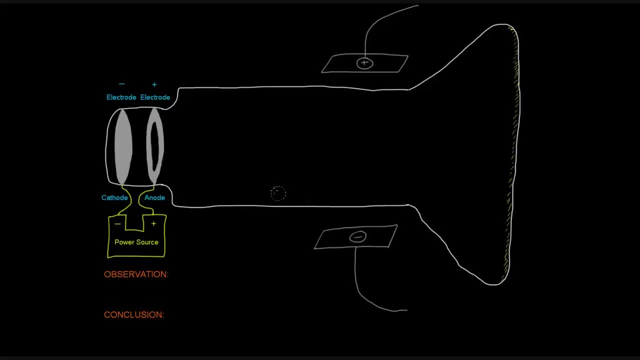 And he wants to see which direction the beam will bend in. So he checks it out and he sees that the ray bends towards the positive plate. The ray bent towards the positive plate. So what was the conclusion there? Well, if something, If this beam is attracted to this positive plate, then it must contain a negative charge. 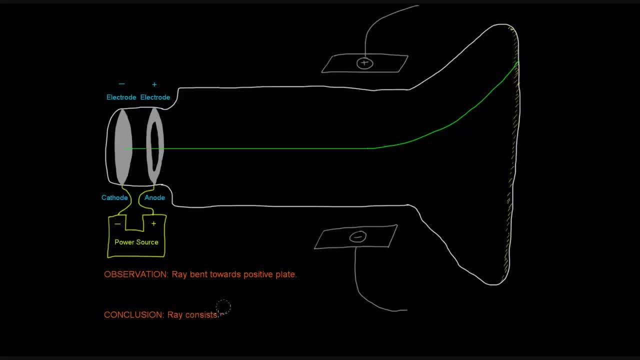 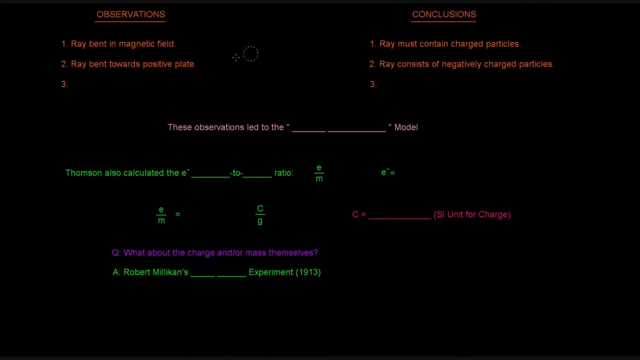 Right, Because opposite charges attract. So his conclusion was that the ray must consist of negatively charged particles. Okay, So then what? So there were a few different observations that he made, a few different conclusions that he drew from them. So we already said that the ray bent in a magnetic field. 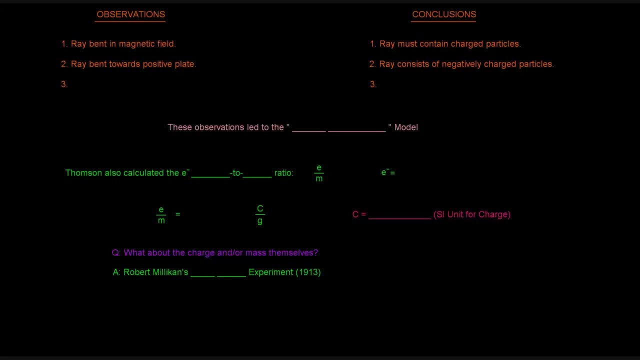 So that led him to conclude That the ray must contain charged particles. right, So there was something charged in the beam, And then he noticed that the ray bent towards the positive plate, which meant that it must have negatively charged particles, specifically, 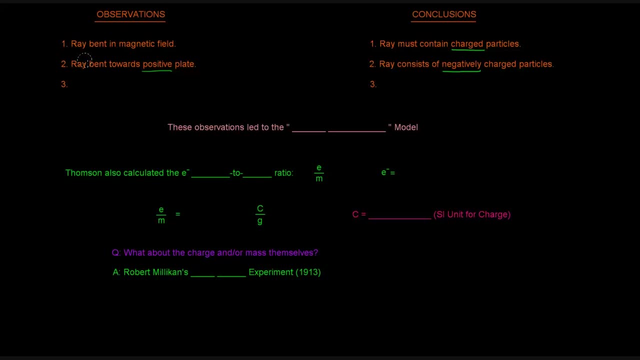 Right, And then what he did was he switched out the metals that he had in the cathode ray tube. So he did it for a bunch of different metals, And what he found Was that the ray was identical For all different metal cathodes that he used. 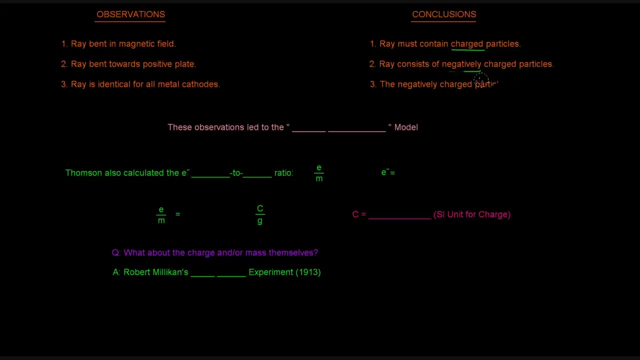 So his conclusion there was that the negatively charged particles are in all matter. Okay, So we have these negatively charged particles and these negatively charged particles exist regardless. The beam being- Excuse me, the ray is identical for all these different metal cathodes. 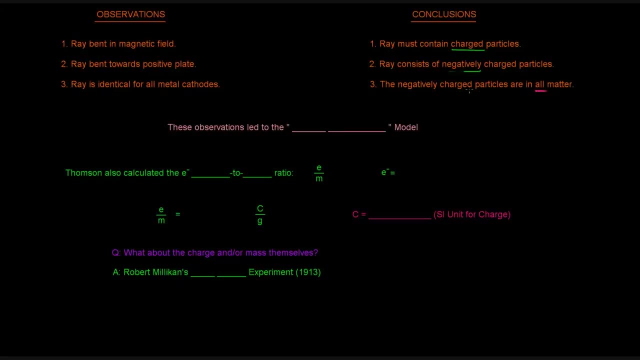 Which that means that these negatively charged particles exist in all matter. So he combined That, That, That these different pieces of knowledge, as well as the fact that these negatively charged particles, which he called electrons, by the way, He called them electrons. 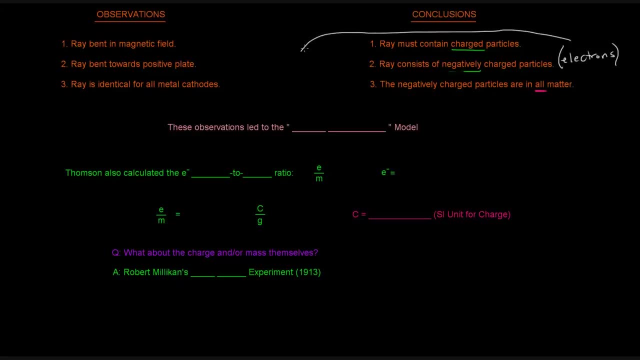 He combined that with knowledge that these electrons Were about One thousand times Smaller than the smallest atom that was known Right, Smaller than the Than a hydrogen atom Right, Which is the smallest atom, Which meant That there is something smaller than an atom, thus disproving Dalton's model right. 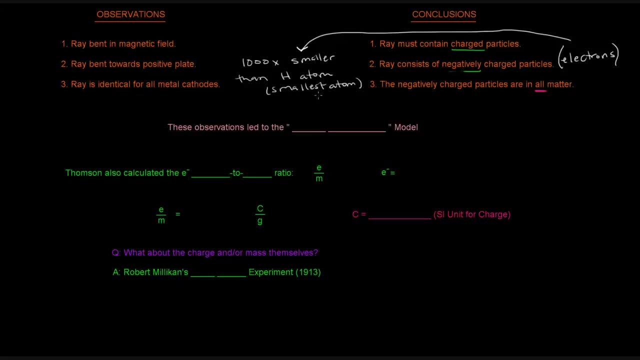 Of the billiard ball model. Because If He says in one of his postulates that Atoms are tiny, Indivisible particles, Right It will. If there's something, these electrons namely, and they're a thousand times smaller than the smallest atom, then there must be some. 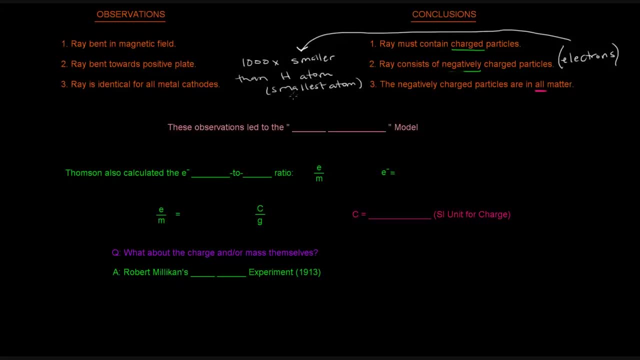 Then that means atoms are divisible into subatomic particles, Right? So these observation, These observations led to what was called the Plum Pudding Model, And we'll talk about the details of that in, actually, the next video. Okay, So that'll be in the next video. 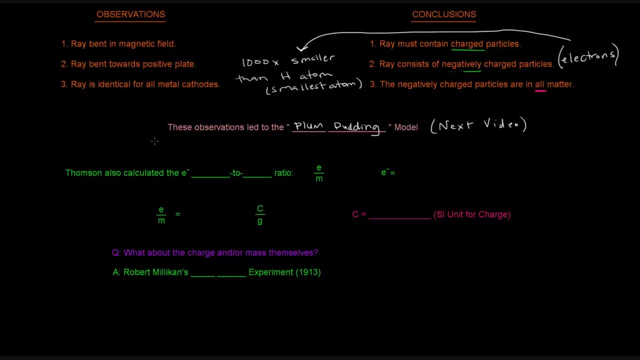 We'll see what that looks like. Thompson also did. What he also did was he calculated the electron's charge-to-mass ratio. Okay, So this little E with a superscript, that's a minus sign that represents the electron, Because electron, of course, starts with the letter E and the minus sign indicates a negative charge. 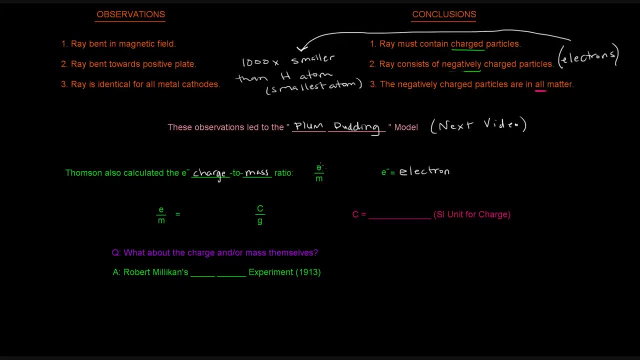 So he calculated the charge-to-mass ratio, which is E over M, Okay, And Where E, specifically, is the magnitude of the electron's charge, Because the actual charge of an electron would be negative, E Because electrons are negatively charged. 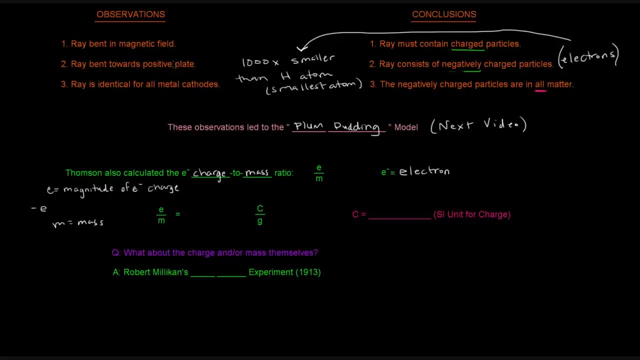 So, and then of course, M is the mass. So the ratio between the two he found to be 1.758821 times 10 to the 8th C per G. C stands for G, C stands for coulombs. 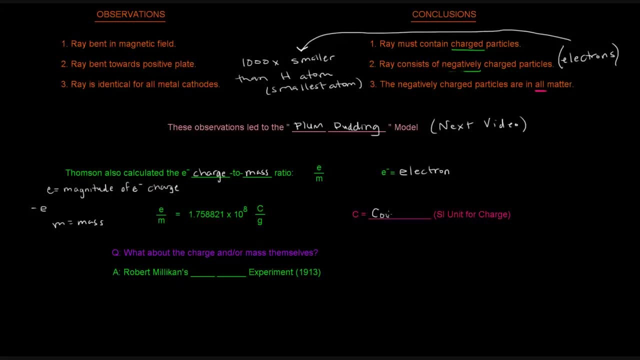 So it's coulombs per gram, And coulombs are basically the SI unit for charge. Okay, So now what was interesting is that he couldn't actually calculate the charge itself or the mass itself. Right, He couldn't calculate either one. 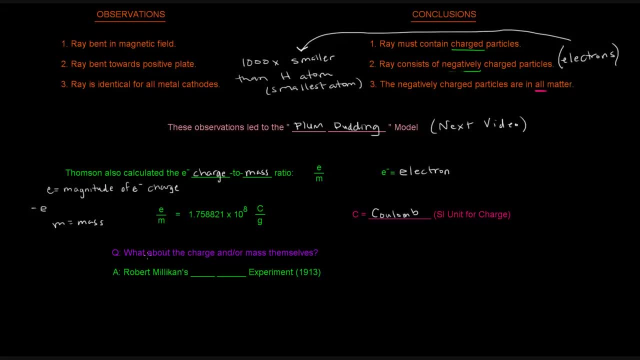 So he calculated the ratio, Okay. So the question is, what about the charge and or the mass themselves, Right? Well, Robert Milliken's oil job experiment kind of reveals the secrets of that question. Okay, So we'll see that in a future video as well. 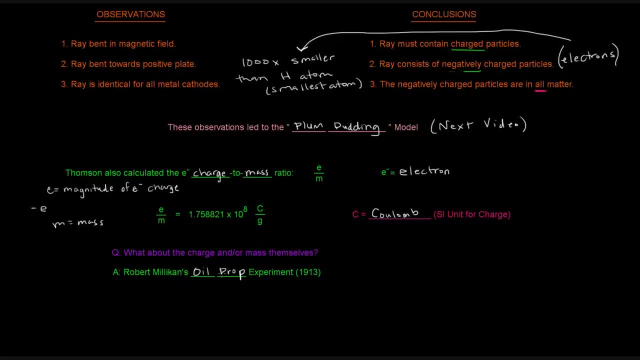 Hope that video was helpful in kind of understanding the cathode ray tube experiment. Definitely be sure to watch the plump pudding model video to make sure that you understand what's going on. as far as the development from Dalton's model to this new model, 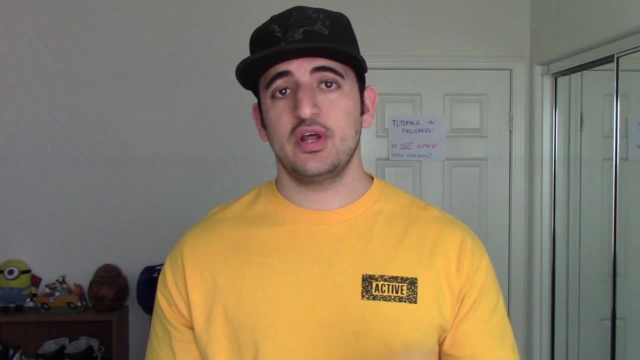 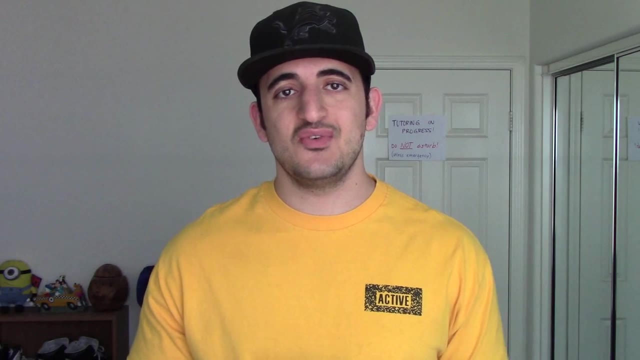 Thank you for watching. If you found that video helpful, be sure to hit with a like and subscribe for more content. Also follow MOVE University on the different social media links in the description below. Thank you and happy studying.